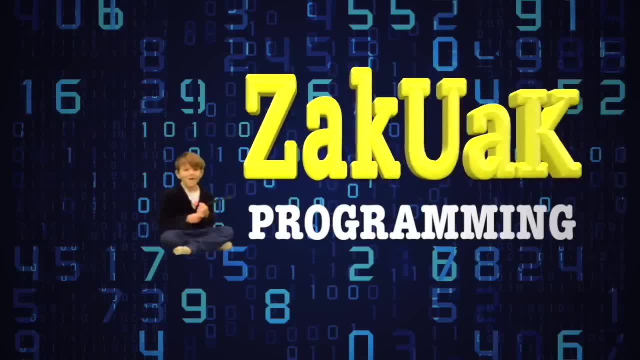 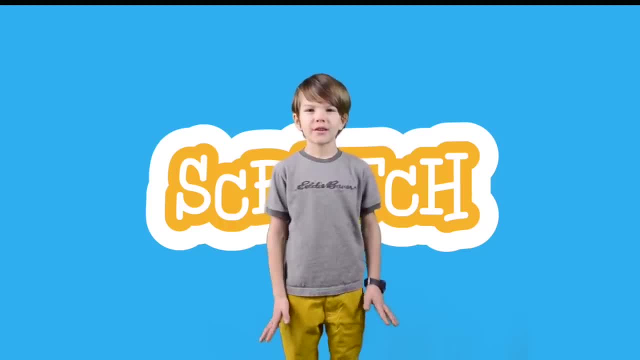 Hi guys, it's me, Zach Ulach, and I hope you're ready to start real programming, because today is our video in real programming and we're going to be starting off from scratch. Scratch is probably the most known programming language for children and it is especially 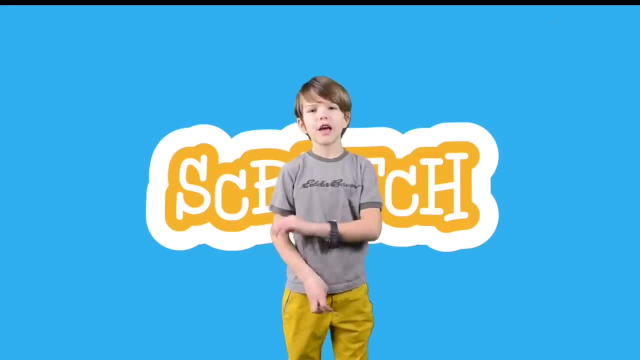 designed for ages 8 to 16, but almost every age uses it, And millions of people around the world use this programming language, including in schools, libraries, homes and community centers. With Scratch, you can program your own interactive games, animations and other. 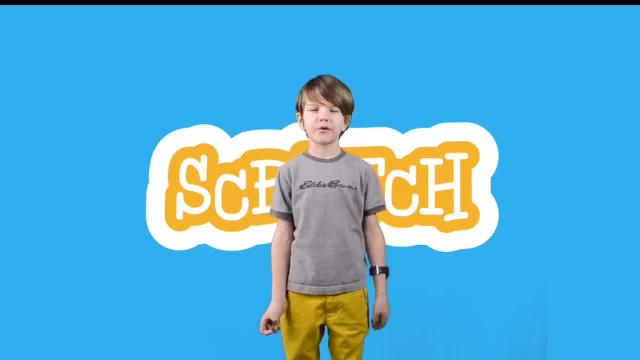 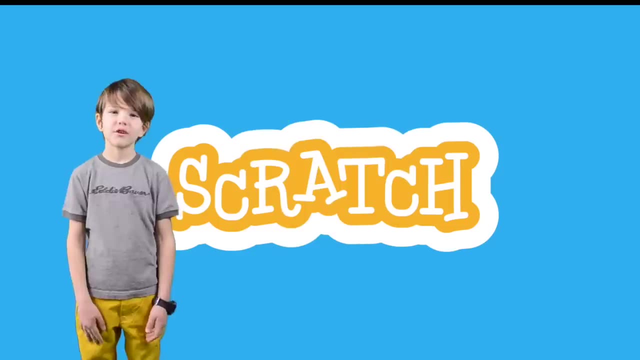 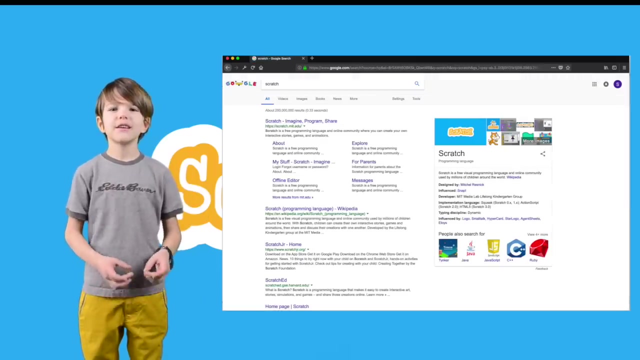 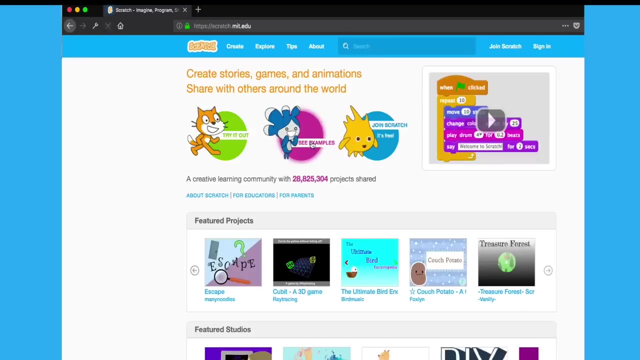 things and share your projects with other people around the world. So let's go. Here's the Scratch website address. Or you could also just type in: scratchcom. And here's how you spell scratch: S-C-R-A-T-C-H. 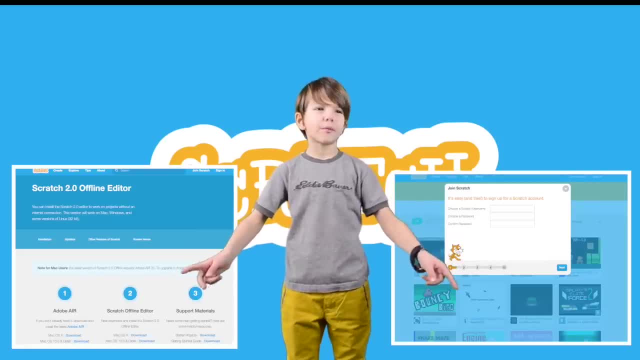 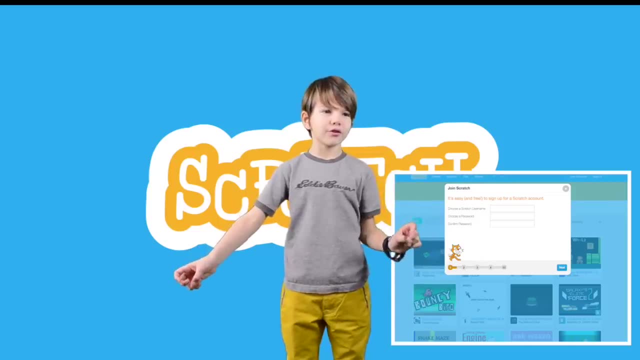 So here are the two options of how you can program on Scratch. The first one is you can program online, but you'll need to just search it up on Google and then yeah, as I said, like on the links and how to spell scratch. 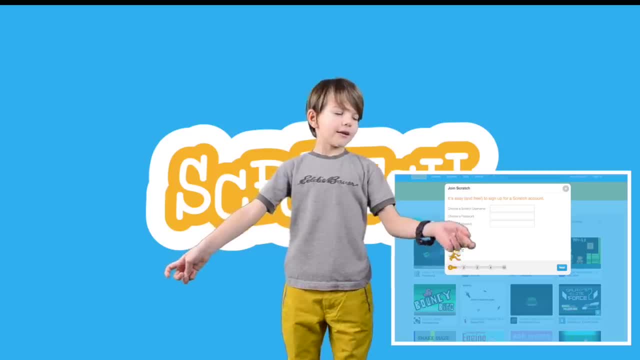 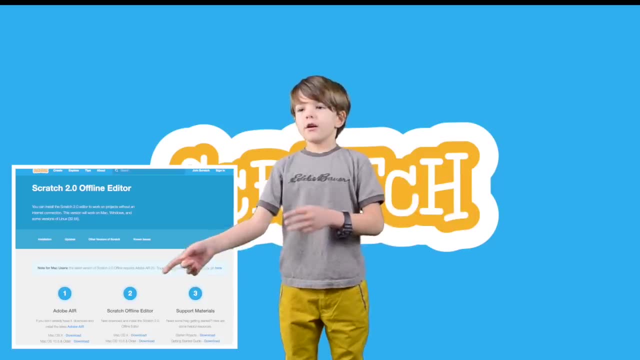 Do that, And then online you have to have the internet. but here's the other version: Scratch Offline. Scratch Offline, you have to download and install the app and you don't need the internet for it. So let's start with Scratch Online. 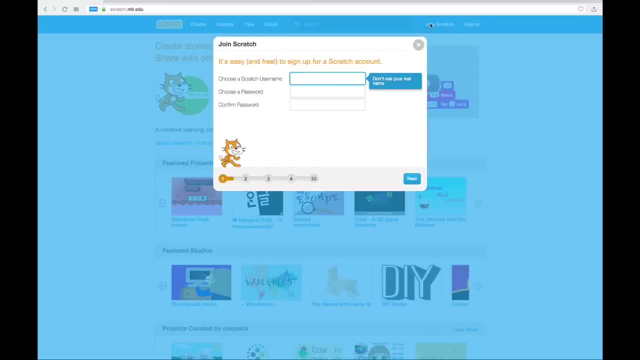 Click Join, Scratch, and then you'll see the form that you have to fill in. Then you'll need to fill out. Next, Your username can be anything, but if it comes up to you that the username already exists, then just pick another username. Then remember the password and type it in. 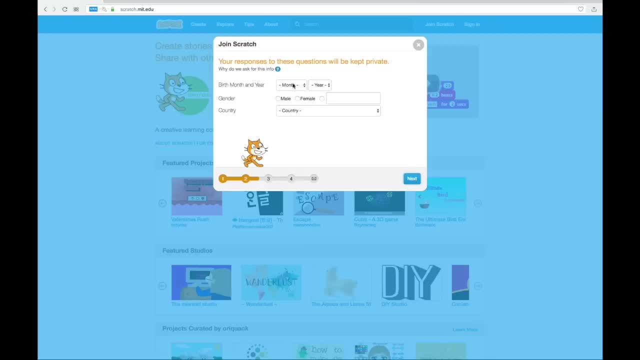 Then press the Next button. Next you have to do your birthday and pick and pick your gender and your country depending on your age. it will. it might ask you your, your parents email, so you, you should. so please have your parents with you and and tell. 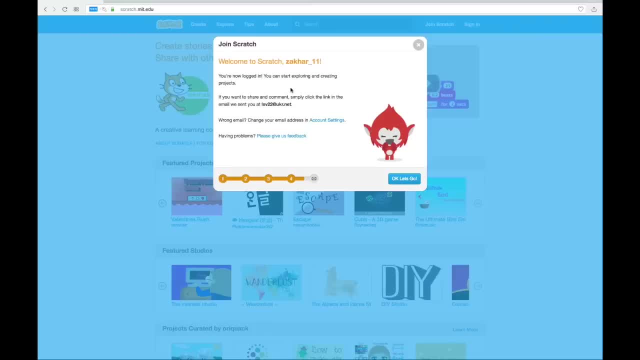 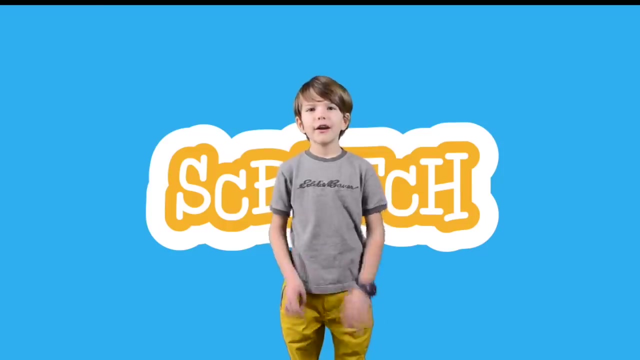 them to type in your their email: hooray, if this screen appears, join scratch, then you're ready to program in scratch. so when the screen appears, just click ok, let's go. actually i use both versions of scratch, so now let me show you how to download and install the scratch offline and how to use it. 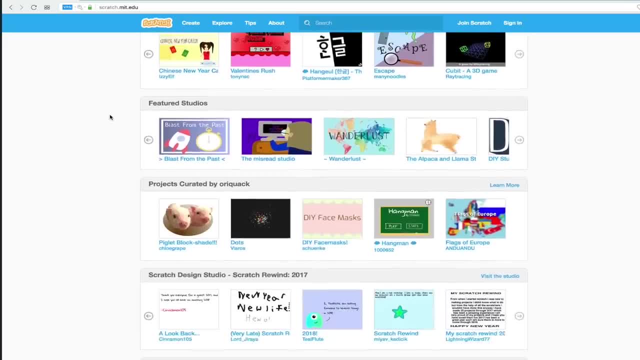 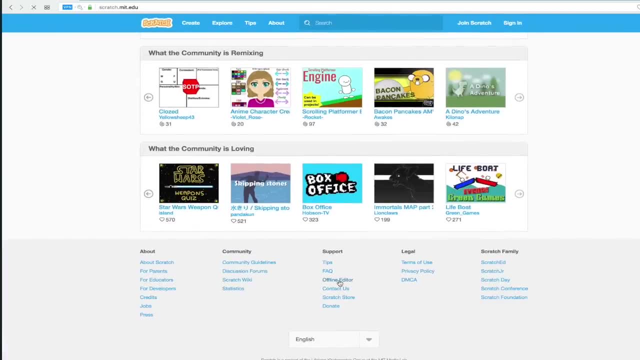 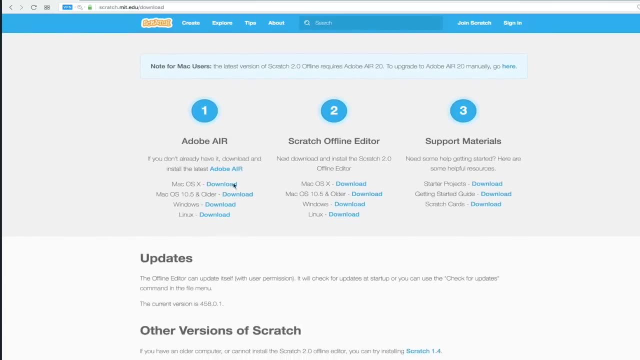 on this main screen, scroll down, and then there's going to be support, and then click offline editor. then you'll see the three steps. first it's going to tell you to update all adobe air if you have it already. it's so, try it, and it's not. 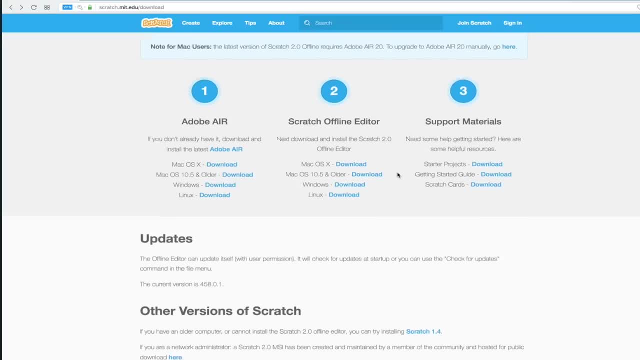 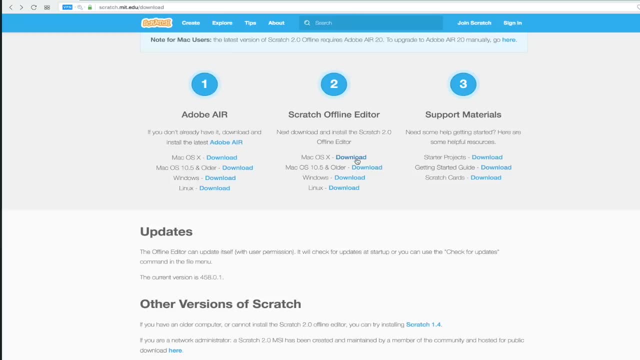 going to be a mistake. next, next, download and install the scratch 2.0 offline editor and then a little lower, you'll see, you'll see the, the version, the versions of the edit of the offline editor. so if you're on, if you're on windows and click the window, then click on the windows download screen. 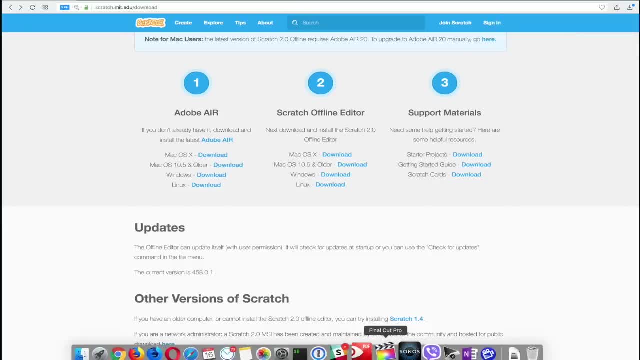 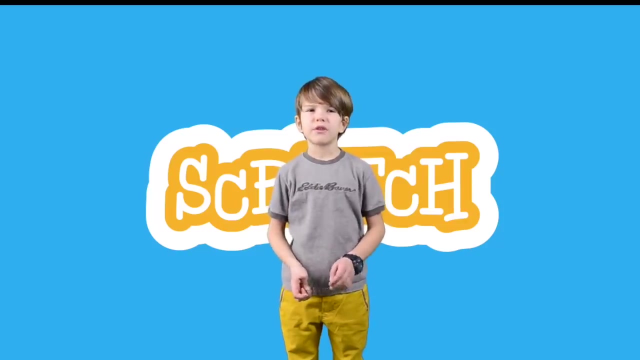 so, as i said, you have to install this and then, when you downloaded and installed it, then run the scratch, then run the scratch offline editor. on step three, you you can find support materials and also the instructions. scratch is actually a real programming language, but here's the difference between like scratch. 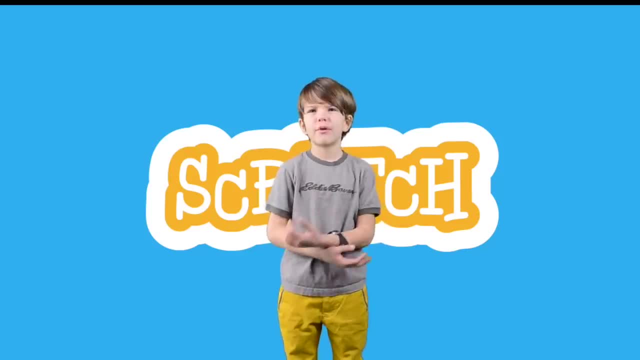 um, here's the difference between scratch and java and python. and like all that in in java and python and all in some other programming languages, you have to type in the words by hand, but in scratch there are really handy blocks that actually mean the same thing. uh, so that that why it's. 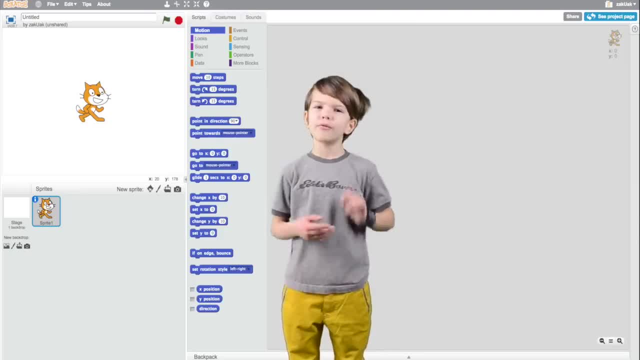 it's made for children. so let's see how a real program looks like in scratch. here's one of the main components in a scratch project. it's called a sprite. here's how it looks like. a sprite can be any object you can. you can draw a sprite. you can pick one from the sprite library. 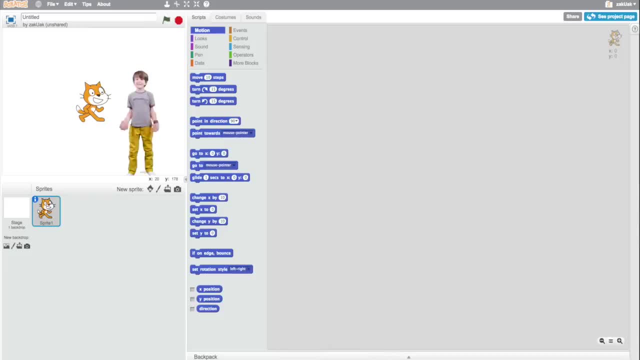 or you can even upload it from your computer. even i can be a sprite. here's another component: the background. a background is actually optional. in our first projects we're not going to use it, but as we go through to the more complex uh projects then you'll see the background is actually a really important part of the scene. the next one: 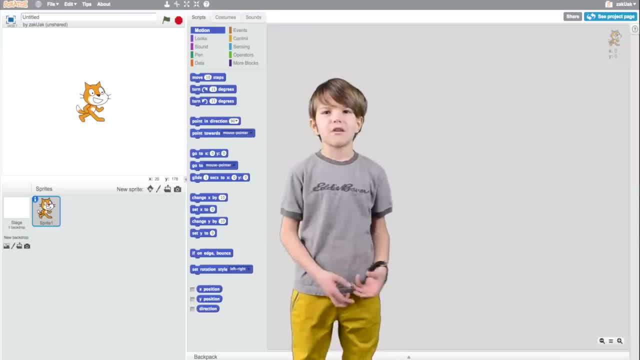 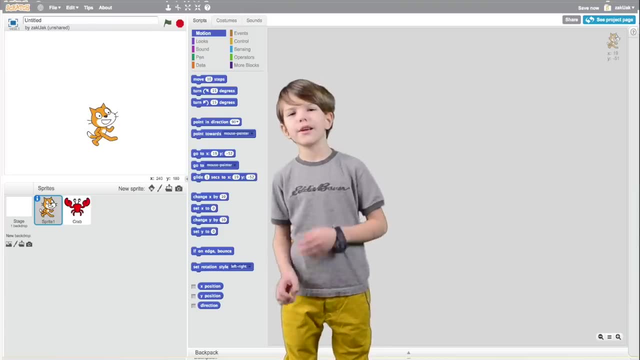 is scripts or or the comments itself. this tells us, this tells the sprite what it needs to do. so what a sprite can do: it can change its look, it can move around, it can play music and it can even speak. they also can react on the keyboard or input on your mouse. they can interact. 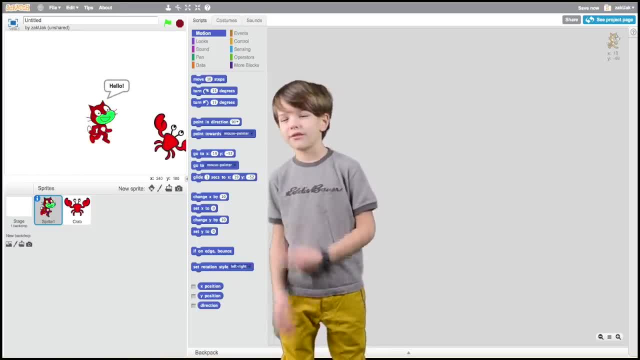 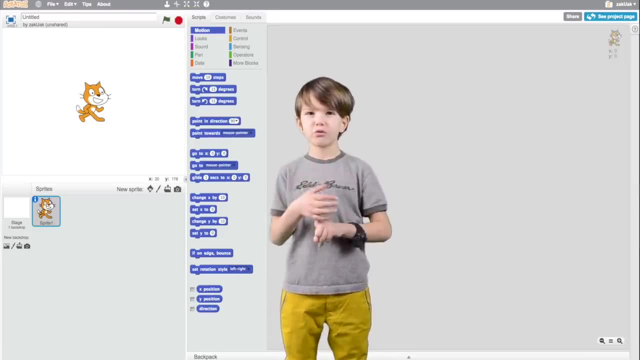 with other sprites. oh, and i'll show you all of that later. so let's look at the command blocks. all the blocks are split in groups like control, motion, event and other. now let's look a little bit how the scratch interface looks. here's the full screen mode. 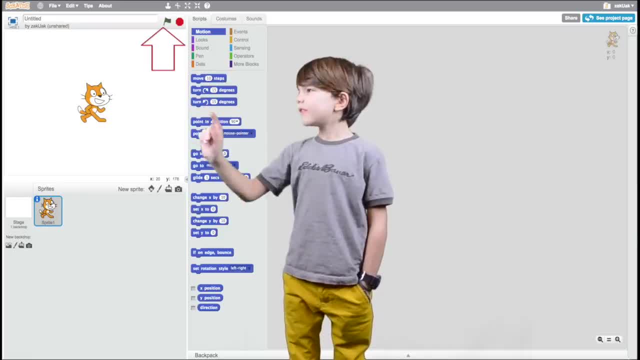 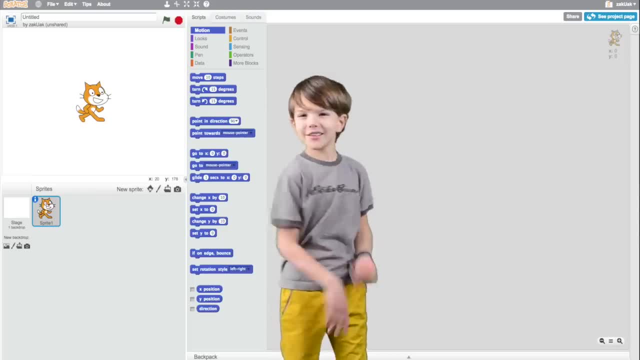 over here you can change your project's name and then the green flag is to start your project and the and the stop sign is to stop your project. but now let's create our first simple program. probably every person who makes his first project would. he would probably write hello world. so let's. 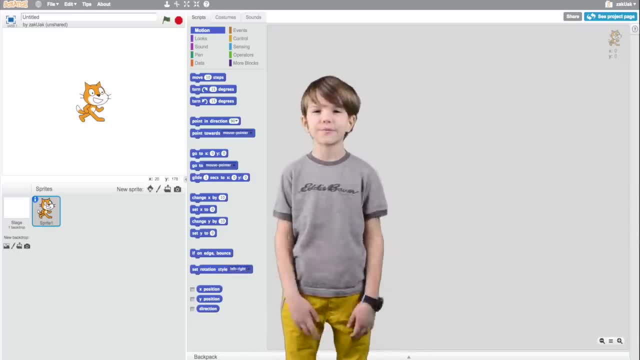 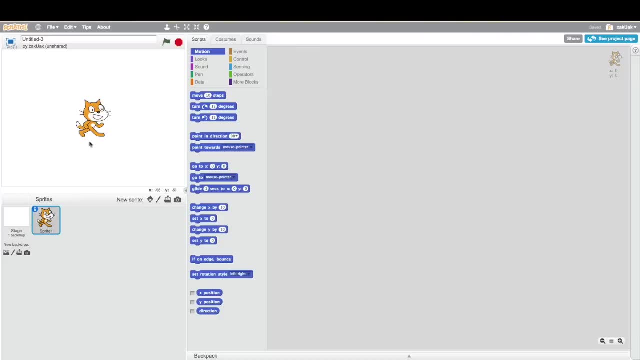 make our first hello world project in scratch. so if you're in the main page of scratch, just click create to create your project. let's use the existing scratch cat sprite with our program. now let's go to the events category and drag and drag the when green flag clicked block to your to your screen. 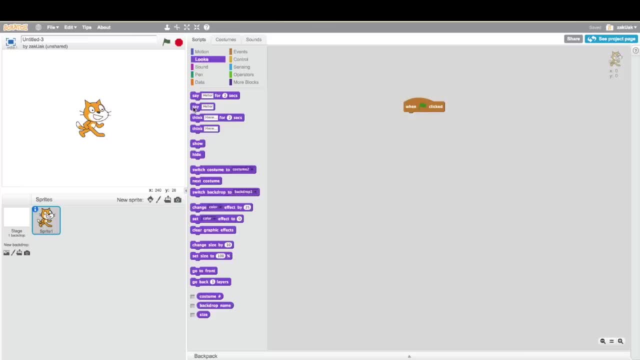 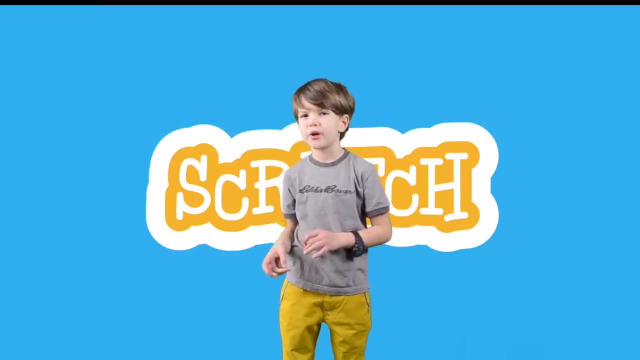 now let's go to the looks category and drag the say say hello block and then change it to hello world done. our first project, hello world, is done, so let's see how it works. let's click on the green flag and, as you can see, our cat says hello world. let's create a more complex programmer game. 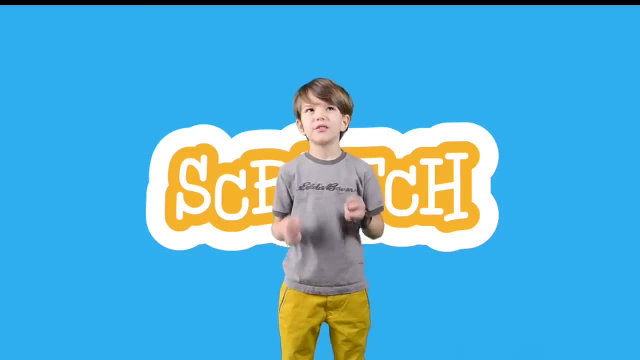 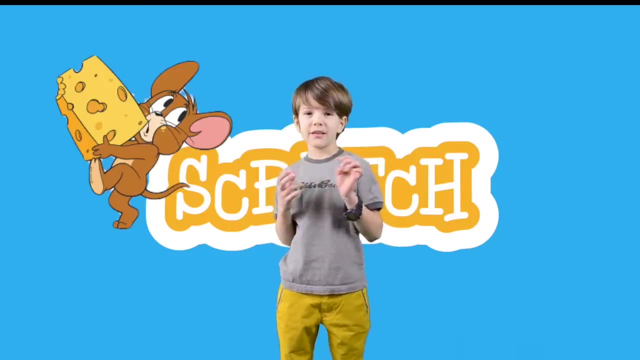 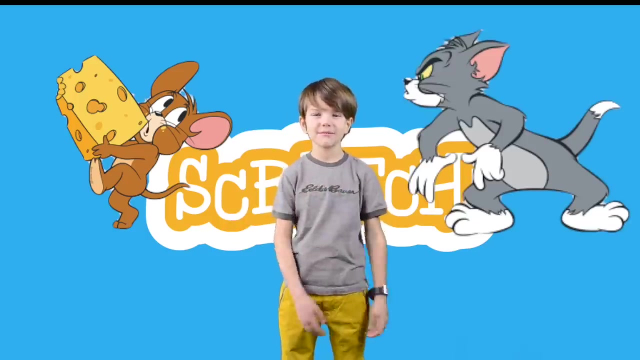 let's make a program that's called clever mouse. the mouse has to get the cheese, but but it, but it has to be careful because they're a cat and and they can, and they can get the mouse. so again, go to the main page and click create or, if you're on the already, 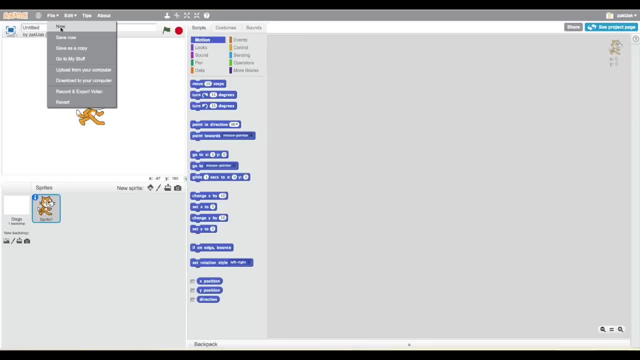 on the project page, then click on file, which you'll find it on the top left corner, and click new. so let's give our project a name and let's call it clever mouse. let's delete the spray and start over to choose a new sprite. if you want to choose it, then click on the 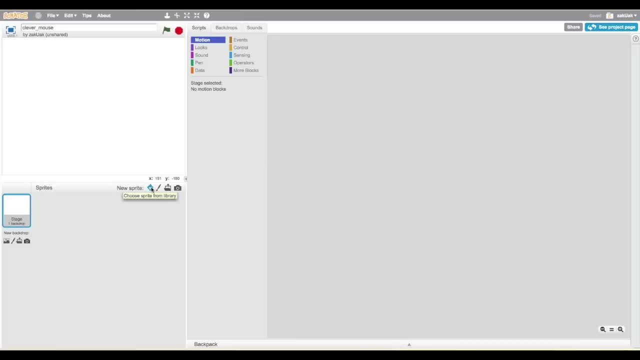 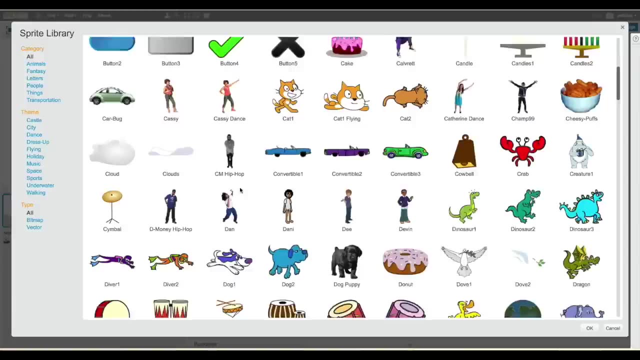 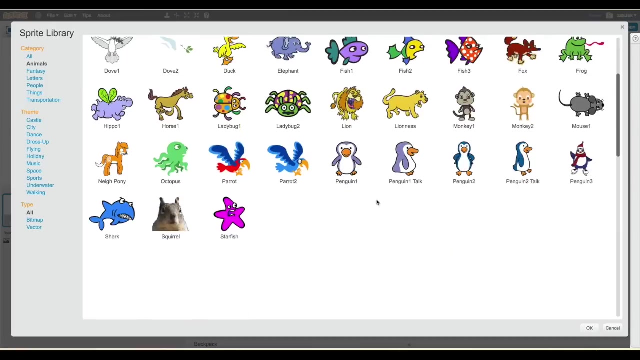 choose sprite from library. so when you go to the sprite library, you'll see a lot of different sprites that are actually in ABC order and they're split up into categories. so let's go to the animals category and let's start off with the mouse. so here's a big mouse for us actually. okay, we have the sprite. 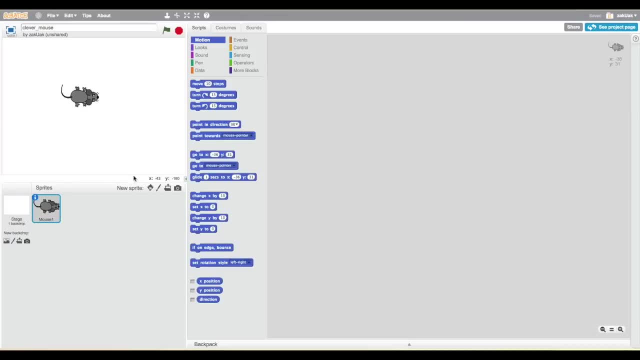 and let's start writing the program. so now let's get the green flag again from the category of events. now let's go to the category control. then let's drag out the block forever. forever is actually a really important block, and and here's what it does. 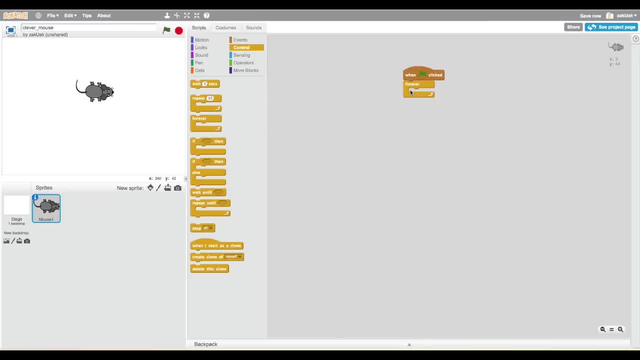 it. you can put different blocks in the forever loop and the forever loop will do, will do this, will do this program forever until you stop it. right now, we are the mouse to complete a program, for it to do something forever. so now let's go to the motion category and drag out. 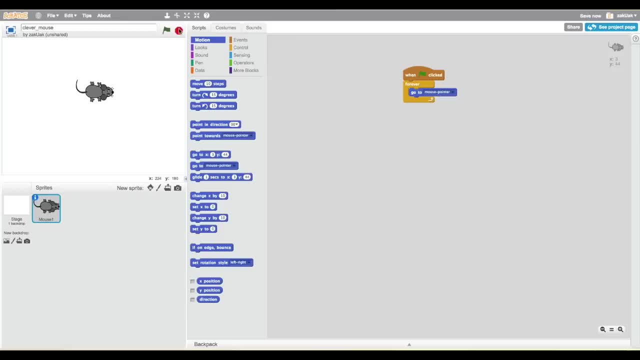 go to the go-to block. the go-to block simply tells the mouse, this mouse, where to go, where to go. so we want it to go to the mouse pointer, which which the mouse pointer, is the our computer mouse. okay, now let's try. let's press the green flag. 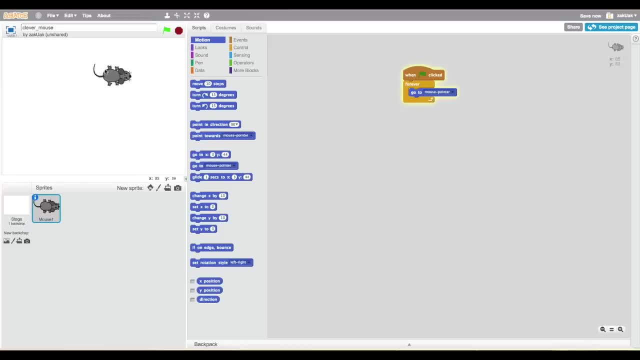 and try and see how it went out, how our little script worked. so, as you see, our mouse always forever goes go, goes with the goes with the pointer of our computer mouse. now let's try to make our mouse smaller. so here's what you have to do to make it smaller: go to the menu and press shrink. it's gonna have four arrows. 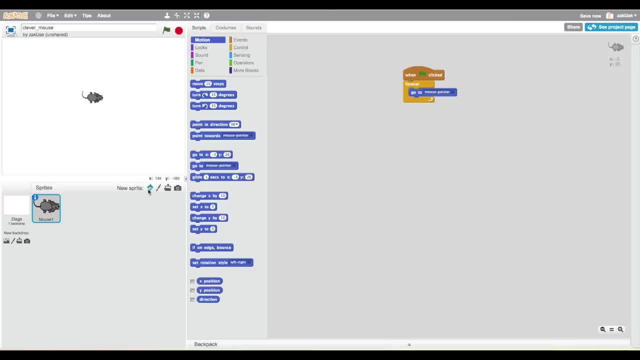 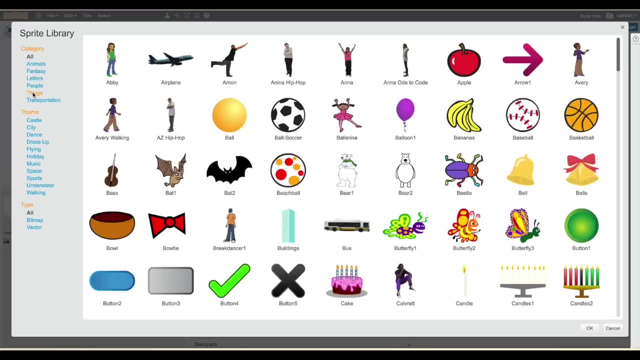 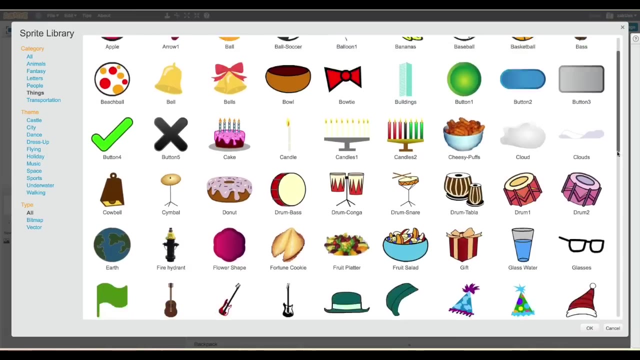 pointing to the middle. now let's make a new sprite. it's gonna be the cheese. it's gonna be the cheese that our mouse has to catch. unfortunately, you can't find a cheese block in the lot in the sprite library, but that's not a problem, you can. 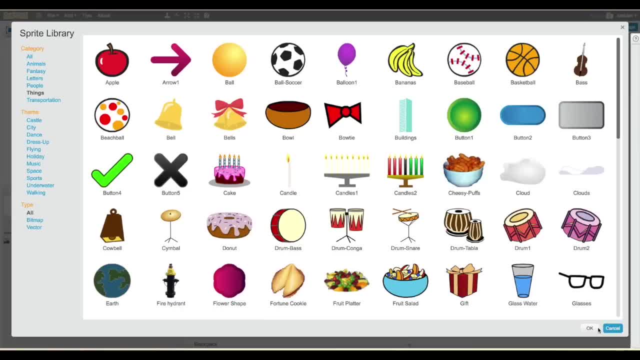 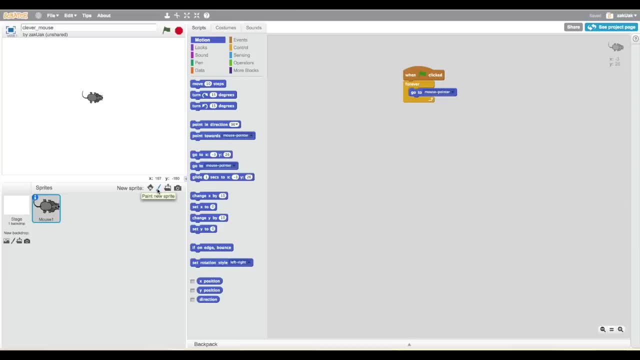 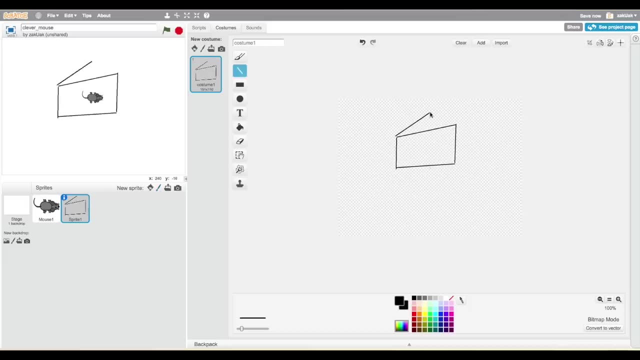 draw it by yourself. so, to start to draw a new sprite, go to the new sprite section and press the second option, which is gonna be a brush. click on the brush and then a screen will appear will appear and you can draw your cheese. so here we're just drawing the cheese. 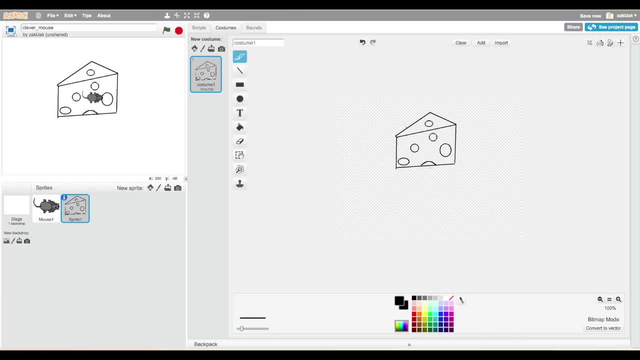 and now let's paint the cheese yellow. actually it's not gonna be seen that hard. you just have to press the, the paint bucket and then, and then, and then press it, click it on, click on the cheese with it and then it will color the cheese. but if, if there's a little space, but between the lines and the cheese, 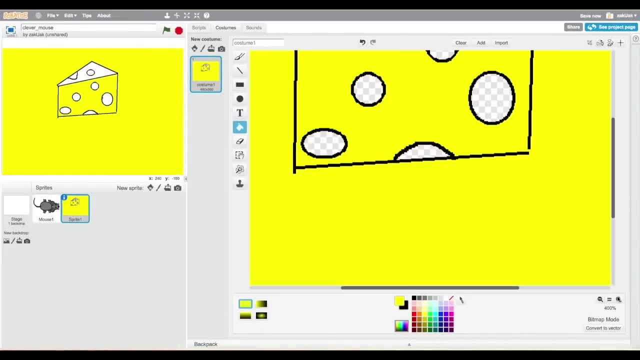 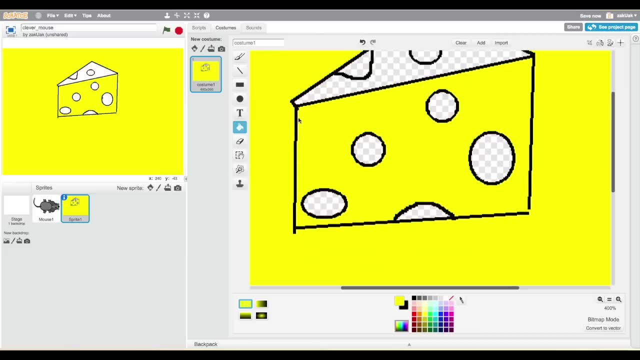 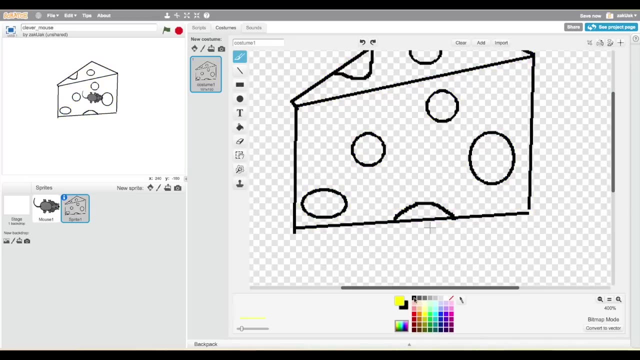 well, not only cheese, like in different sprites, then say, the yellow paint, it will go all over. so now let's fix this. so we, so we don't have like everything in yellow, so we're just gonna zoom in a little bit and then well, and then we'll. 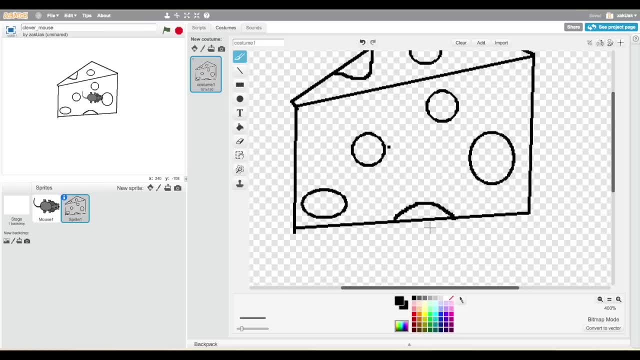 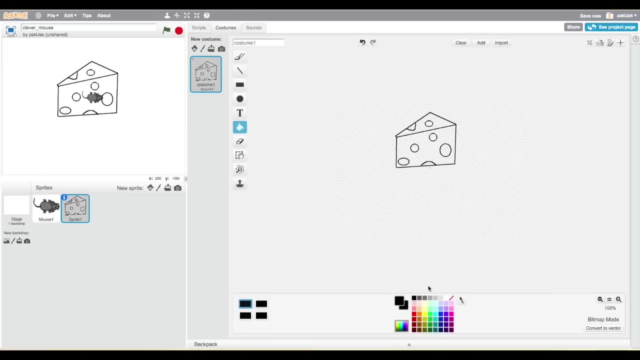 finish the line and also we could erase a like part of the line that's out of the that we don't need you. so please pay attention to the set set costume Center option. it's really important because if you don't have it, you're not gonna be able to paint it. 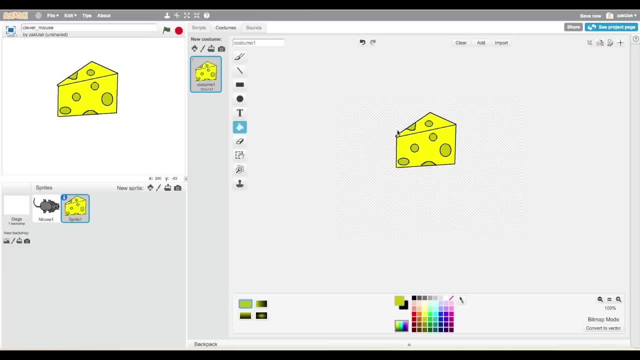 so please pay attention to the set costume Center option. it's really important because if you, if you have a sprite and you don't set it on this Center, it's if you don't set the center. there's gonna be a lot of unknown mistakes because the center is gonna be like anywhere, so your sprite would be in. 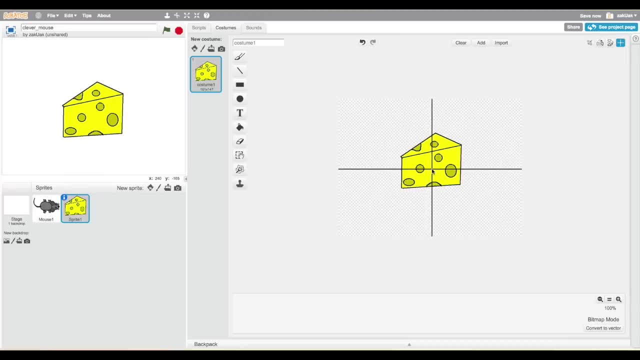 in in places that you weren't expect expecting it to be. so now, since we drew it, you could see it's like too big, so so here's. so here's how we we're gonna shrink it. we can't shrink it with the shrink tool or that I showed you a little earlier, but here's how we're. 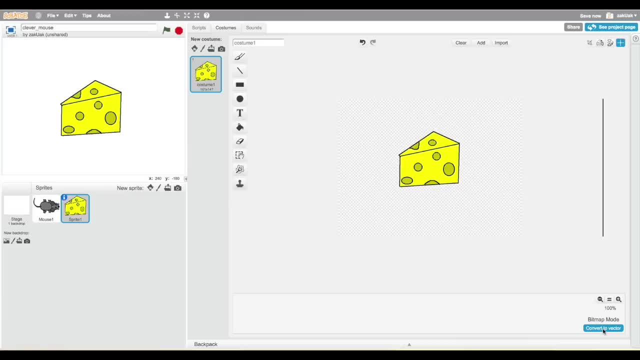 gonna shrink it. we're gonna shrink it by pressing. you'll see, on the bottom right corner bitmap, bitmap and vector. so prep, so press convert to vector and then and then click on a sprite and then, and then there's gonna be a square with circles, and then that's how you shrink it. 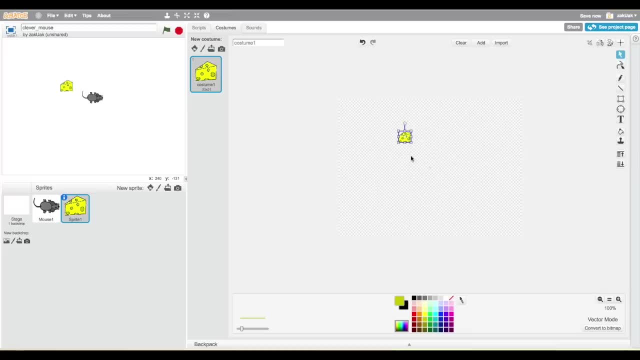 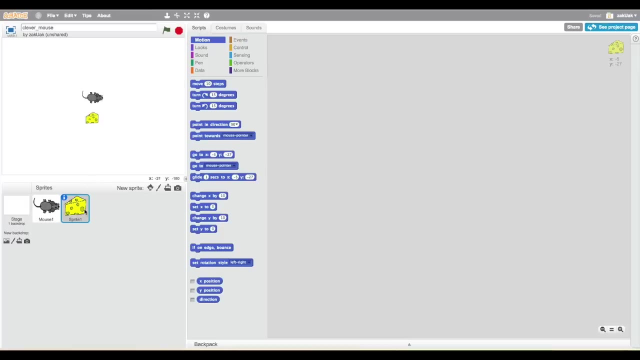 so you can only. also let me tell you that you can only make the program for one sprite, so so on, so on the sprites. on the sprite section there's gonna be your sprites that you have, so so click on the sprite that you're, that you're trying to. 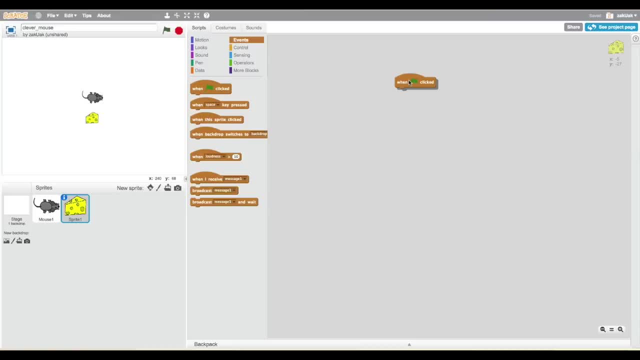 program and it's gonna be highlighted in blue lines. so that means that you're that you're programming that sprite. so let's program the cheese block. now let's change the name of our sprite. let's make the name into mr cheese. so now let's try to hide the cheese, like hide it from the from the page, like 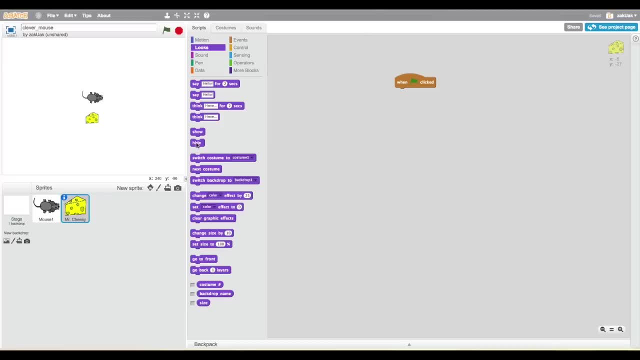 screen. so we're gonna get dragged in, the one green flag clicked, hide and wait, and then we'll wait a couple sex seconds. so well we now we need to make it show where no one knows where it's where the cheese is gonna be, so that so we're. 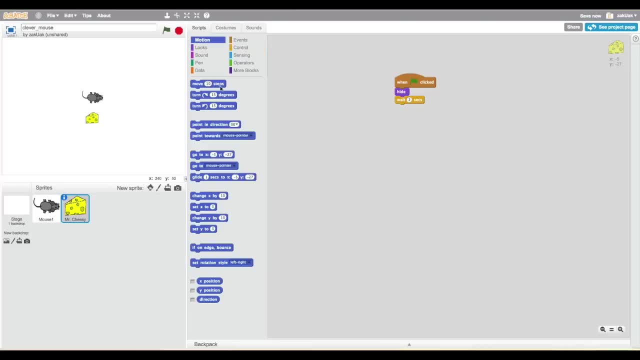 gonna use the pick random block. so here's how we're gonna use it. we're gonna use it with the set X and set Y, or set X, set X, Y, 2, so we're just gonna put in the set random block and in there, and then it will set a random place for. 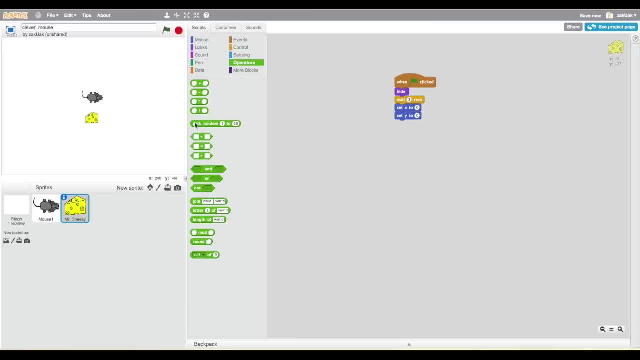 it, but so I'll tell you more about the random- the random block later, but but but so. so I'll tell you more about the random- the random block later, but but so. So we know right now, the random block is for something to appear in random places. 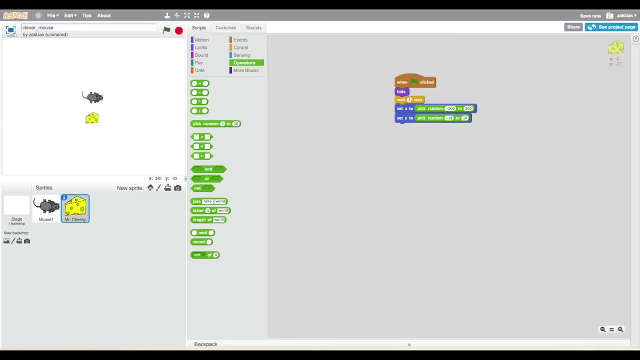 So we're going to find the random block in the category for operators. Okay, let's see how it works. Let's press the green flag. Okay, okay, okay, we're waiting two seconds. Oh wait, I forgot something. 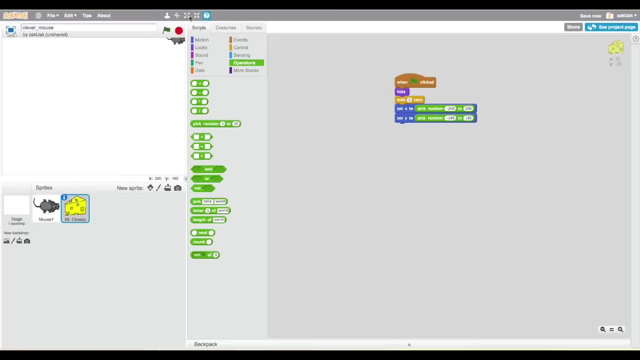 We have to make it show. We didn't do that yet. Let's go to the looks category and then drag on show. Let's try out now and see how it works. I think it's going to work. Good, it works. 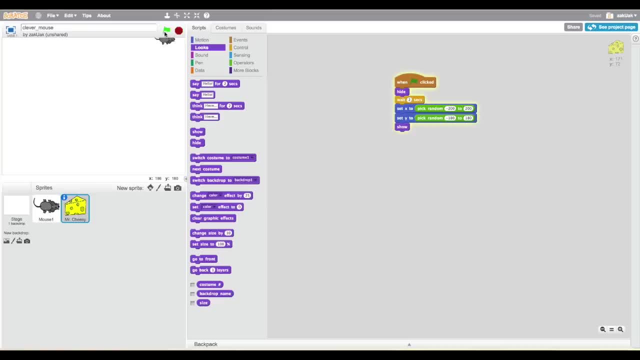 Now let's. Let's see if it's going to go in random places. Yes, now let's try out another time. Yes, it worked. Now let's add a little program to the mouse. Let's make it say like, for example: yay, I got it. when it touches the cheese, 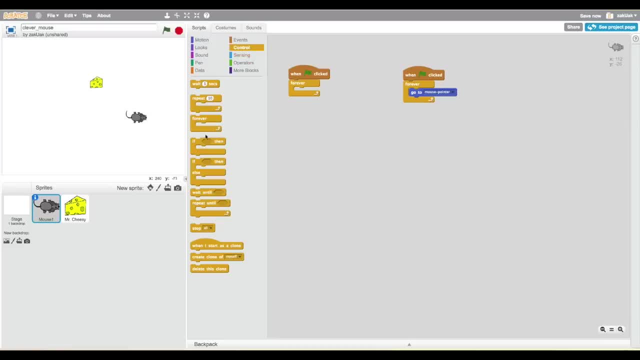 Now let's use a new little block. It's kind of like a. it's actually the shape of a forever loop, but it's going to tell us: if something happens, then do something. In our case, we're going to make, we're going to do if, if touching Mr Cheesy, then say: 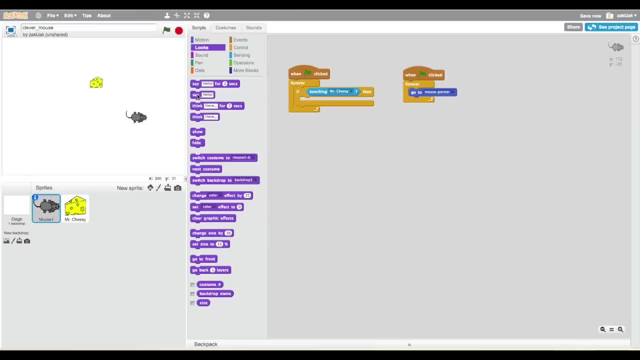 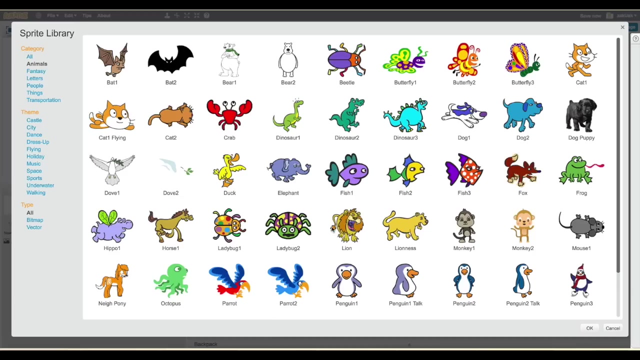 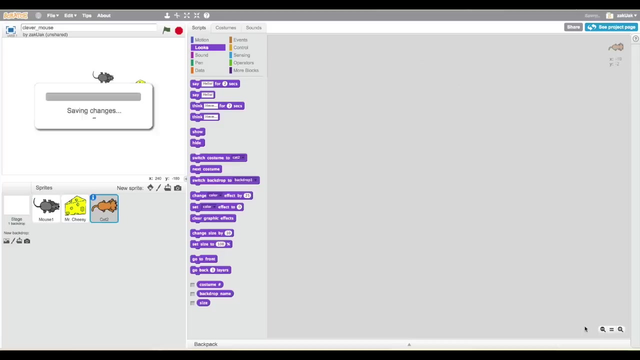 hooray, I got it. Now let's add a new spray of a cat, since, since I mentioned, it's going to. it's going to try to chase the mouse. Yes, And now we're going to use a new block, meaning saying point towards. 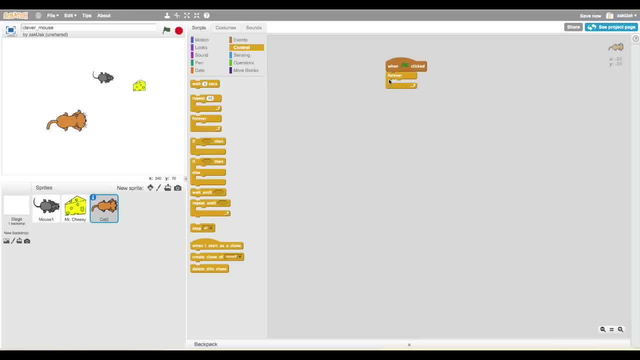 Point towards just simply means point towards something. Well, point towards is to to point, to look in a direction, And don't forget about the forever loop Here. in the point towards block, click that, click the arrow, the black arrow next to the. 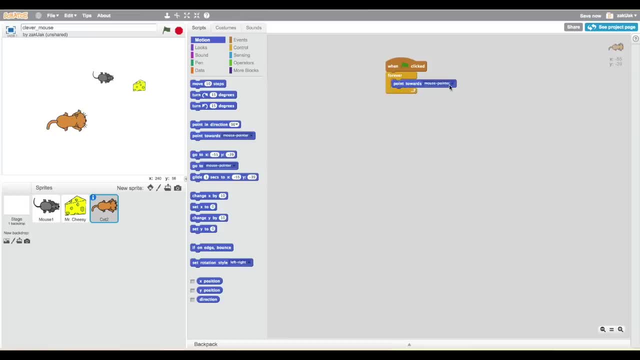 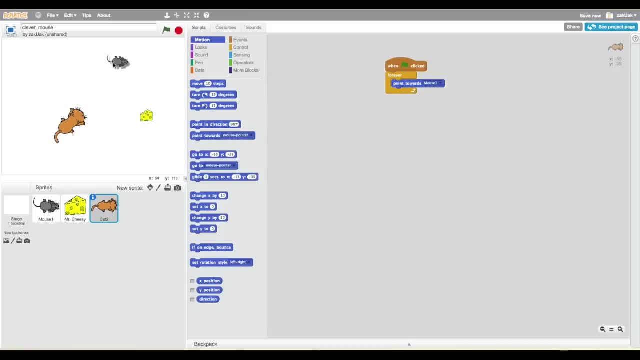 Now let's add another command for the cat to not to not just look at the mouse, but also try to catch it. So we're going to use, Okay, the command block move steps. Okay, let's try. The cat is so fast, it's so hard to do the game. 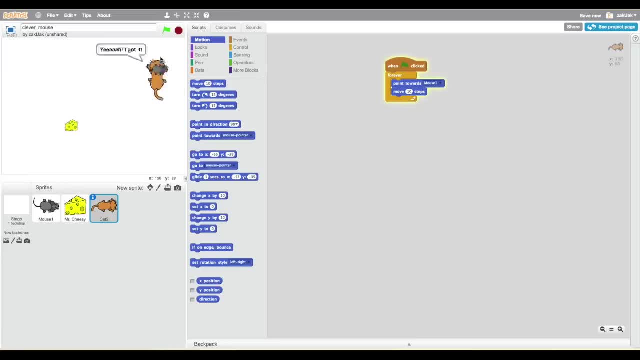 So let's make the cat slower. That's better Now. it's better for the mouse. Now let me show you how sprites can interact with each other. That's actually a little bit. that's actually a little bit harder. It's actually broadcasting. 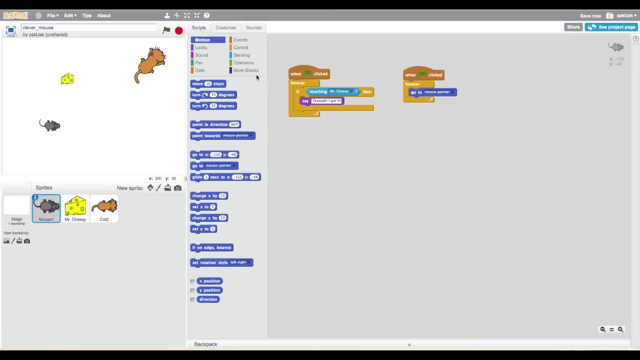 Now we need to do. when the when the mouse reaches the cheetah, it's actually broadcasting. Okay, let's try, If the mouse touches Mr Cheese, for the cat to disappear. That's going to mean that the mouse is winning. 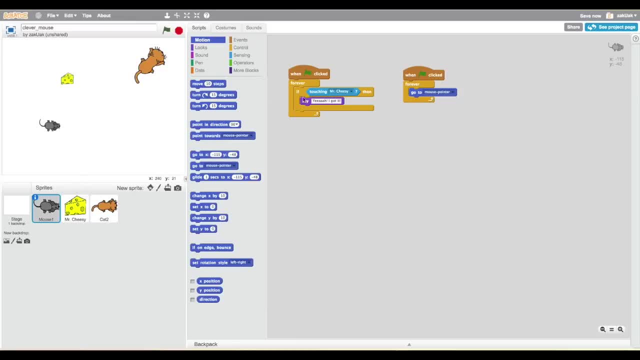 So now let's go to the to the sprite mouse. Be sure, be sure it's, it's highlighted in blue And we're going to add the if, the if-then block. It's going to say, if, if mouse touching Mr Cheesy, then 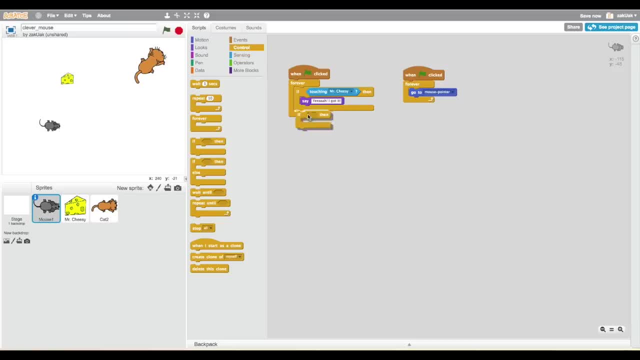 Oh, I forgot. we already have a if-then block. Let's use this block Now. let's add now, let's add the broadcasting part to to the if-then block. Just simply drag broadcast message one to the if-then block under the say: yeah, I got. 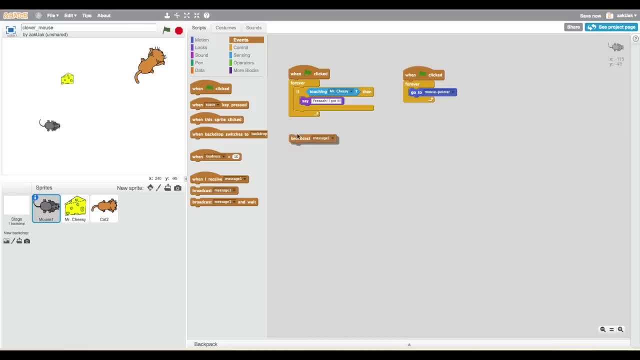 it block And, and, and. as I said, the broadcast block simply, simply creates messages for, for other sprites. Now, let's, let's make a new message, So so where is the message going to go from the mouse? 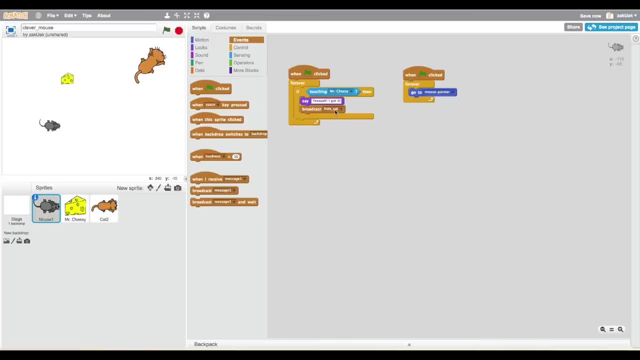 It's going to go to the cat And the and the and the cat is, and the cat is going to read the message and then it's going to disappear. So so we're going to drag the block. when I receive message hide, cat, then dis. then. 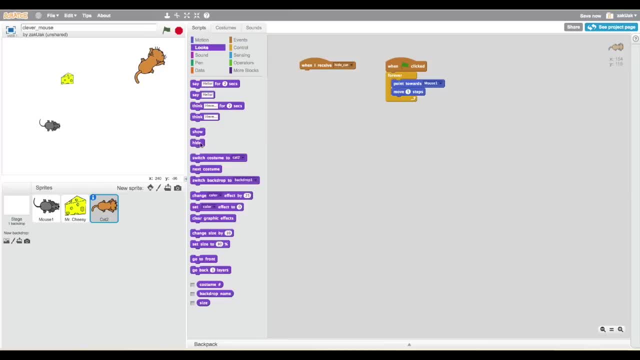 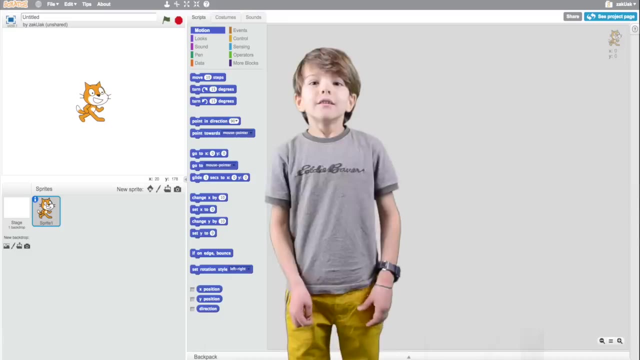 just disappear. Okay, let's play the game. I skipped something in my clever mouse, in my clever mouse project. When I press the stop and then I press the green green flag again, the cat won't show up. Maybe you know how to fix this, how to fix this, but so if you know, then try to do this. 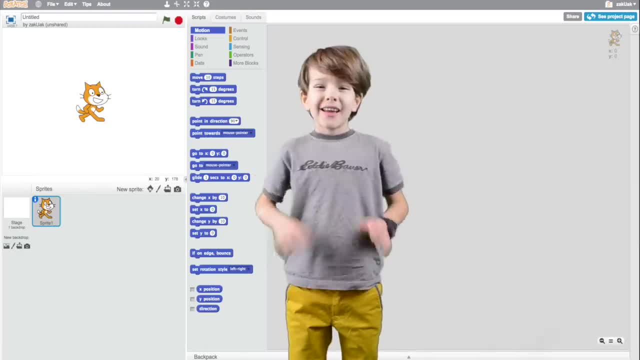 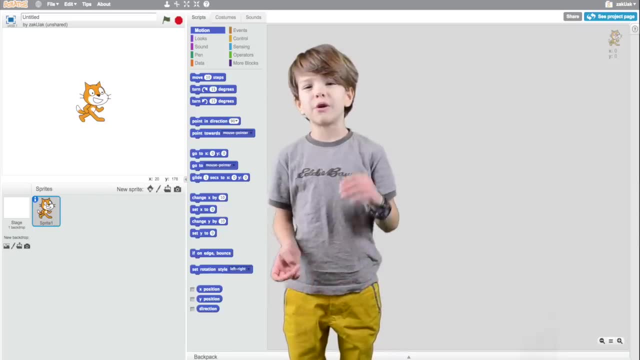 by yourself and write me in the comments, And also maybe you could add stuff to this project. In my next video I'll, we'll, we'll- improve this project and add more, more cool stuff to it. So in this video we learn with you how to start with Scratch. 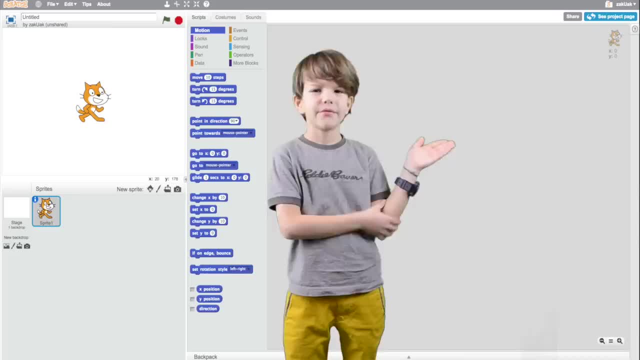 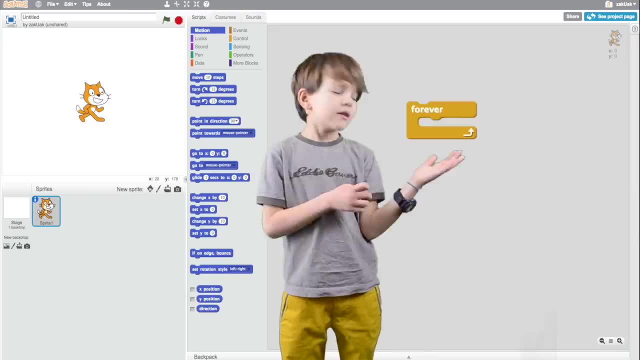 How to make your scratch Like your first hello world program. we, here are the blocks we learned: green flag to start off your project. Another really important block, the forever loop, which simply just tell us the computer to repeat a program all the time. 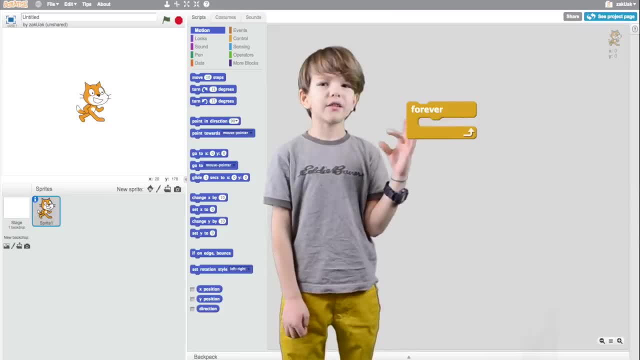 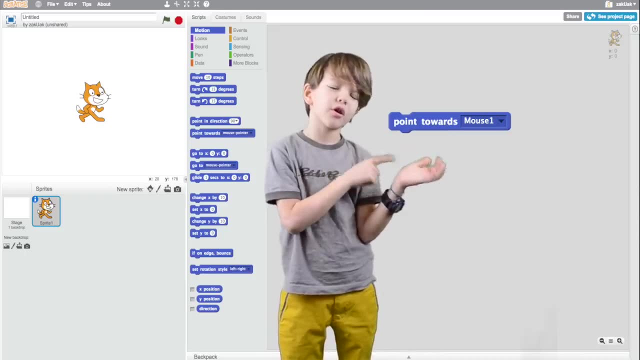 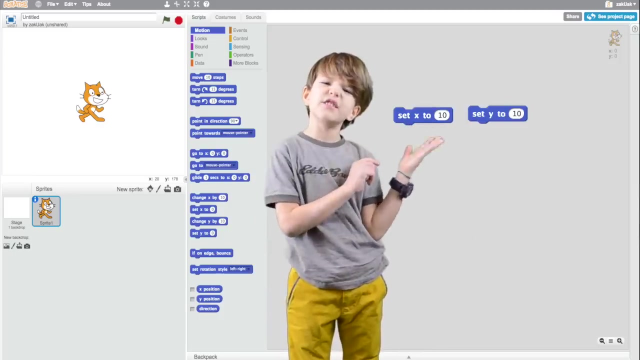 You can put different blocks in there and then and then the forever loop will make the computer repeat this code. We also got familiar This block point towards the height and show command. Just tell, just tell the Sprite in the. just tell the Sprite to hide and show set X and. 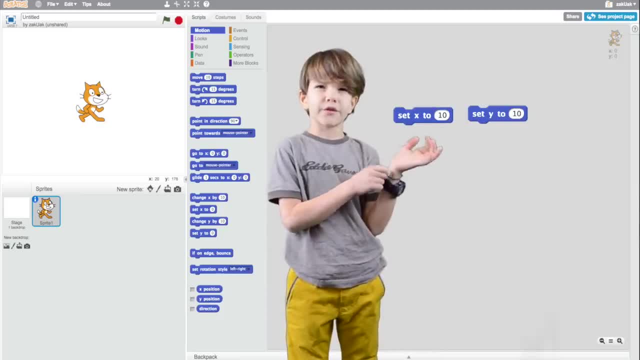 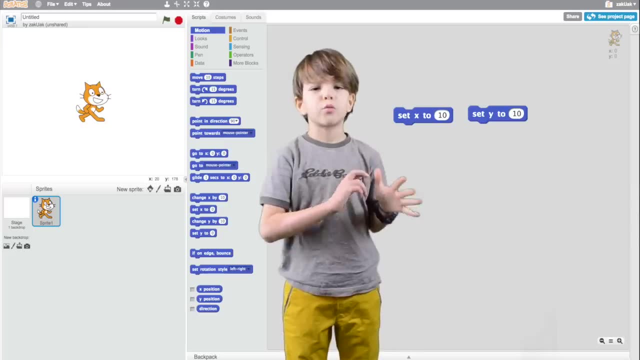 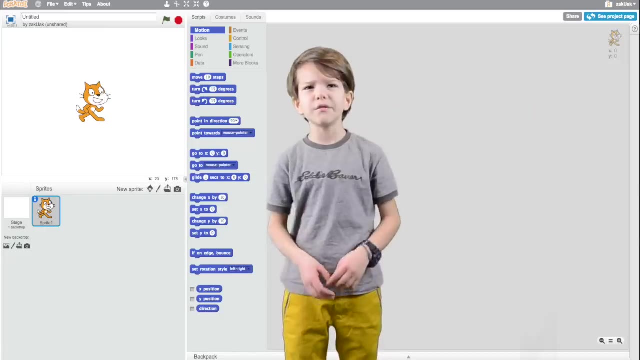 set Y commands mean where the Sprite should be. later on, Well, we'll stop on this X, Y thing and and we'll learn what this actually means, But right now just remember the block. or another really important statement: If something happens, do something. 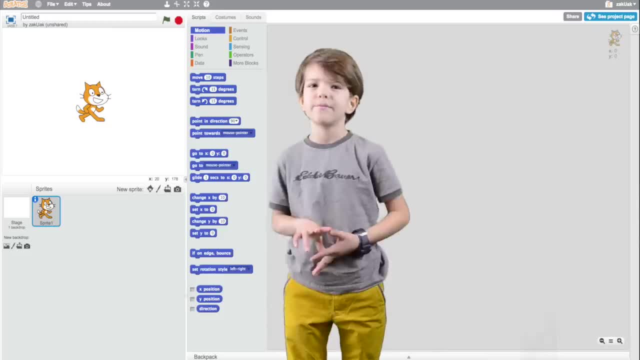 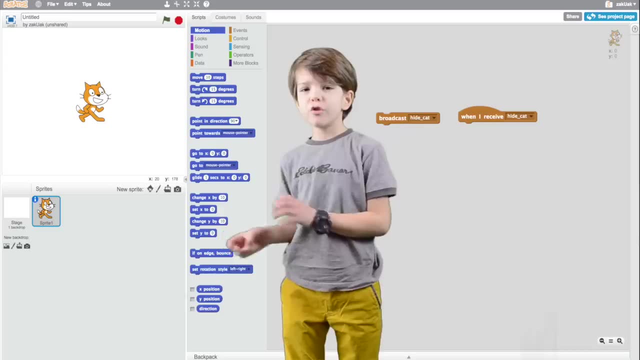 You'll be using this a lot in programming: broadcast. broadcast means a Sprite sending a message to a different Sprite. This is really important and it allows the Sprite to Sprites to interact with other Sprites. So if you like this video, press the subscribe button.